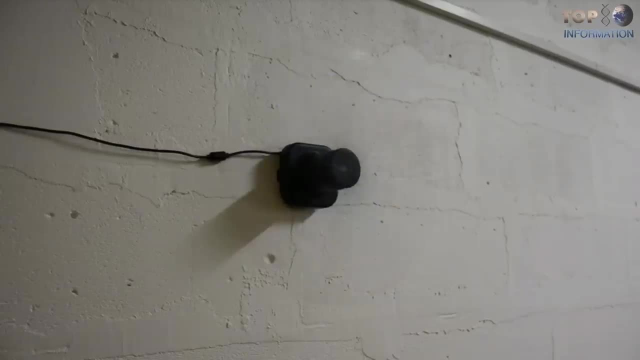 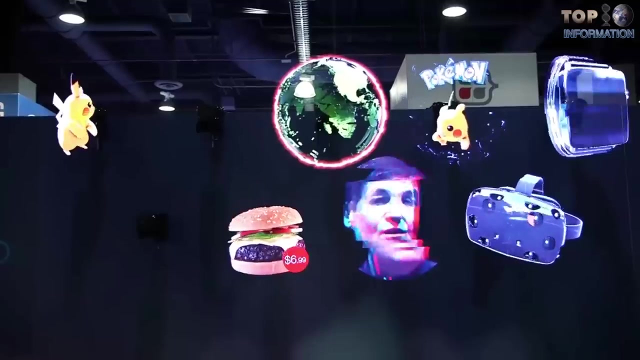 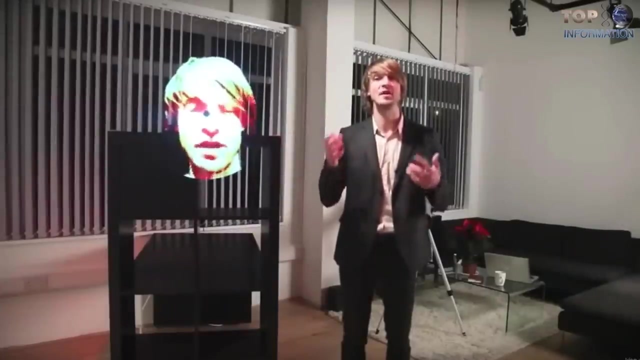 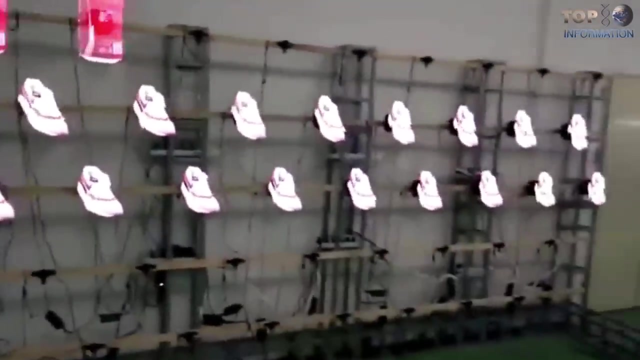 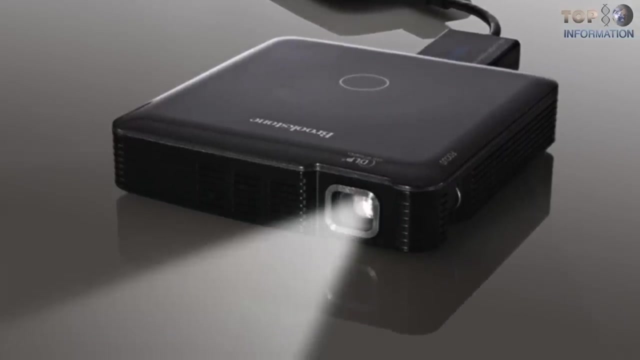 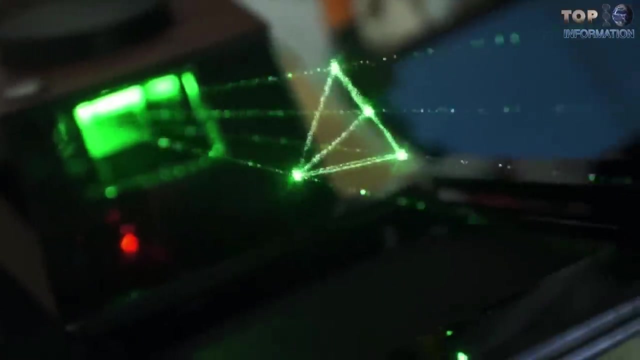 lights On spinning, it produces the holographic illusions. Surprisingly, it provides almost HD quality of holographic illusions. Number 8. Portable Holographic Device. Portable holographic devices are the most compact designs and easy to carry. Scientists from RMIT. 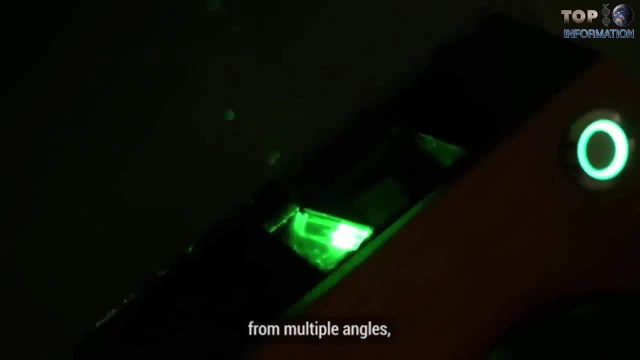 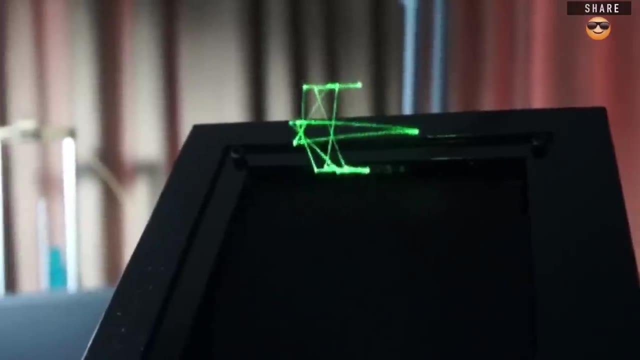 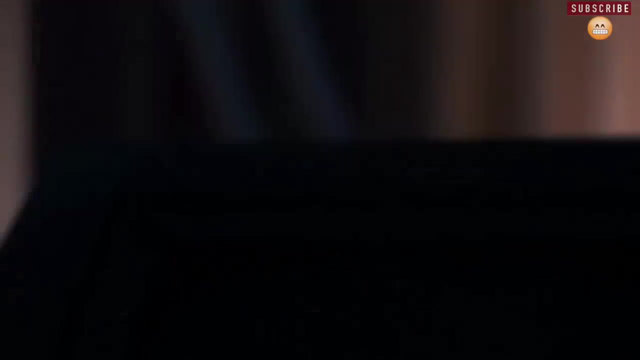 University and Beijing Institute of Technology have invented a portable holographic device known as HoloVect. Surprisingly, it's the world's thinnest hologram, or simply put, it is a thousand times thinner than human hair. This mid-air hologram is visible without wearing any. 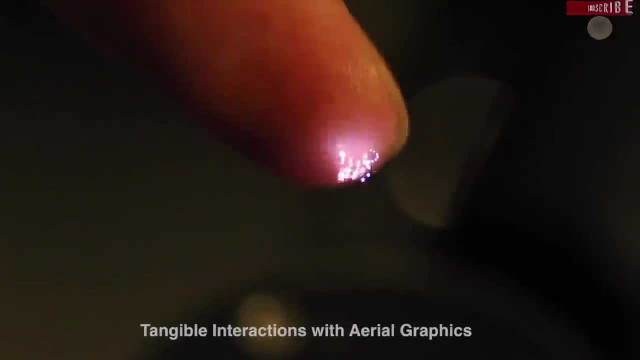 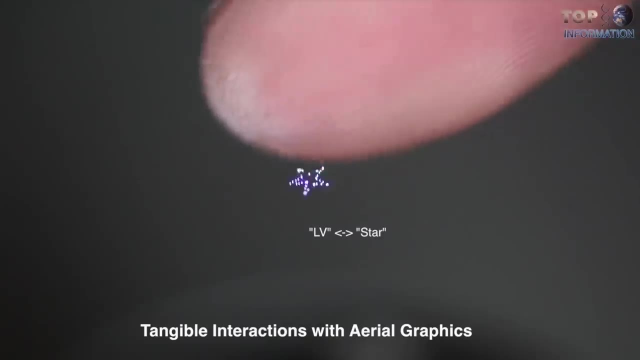 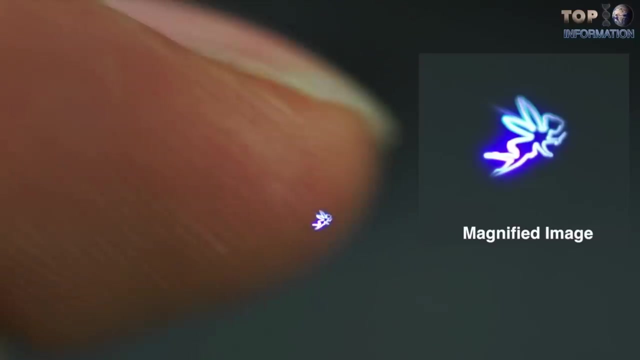 special glasses. That's so cool. Another fantastic portable holograph is Fairy Light. That is an interactive light. Not only can you touch it, but you can also feel it. Four Japanese universities collaboratively developed this tangible aerial volumetric graphics, And this technology uses femtosecond lasers that are capable 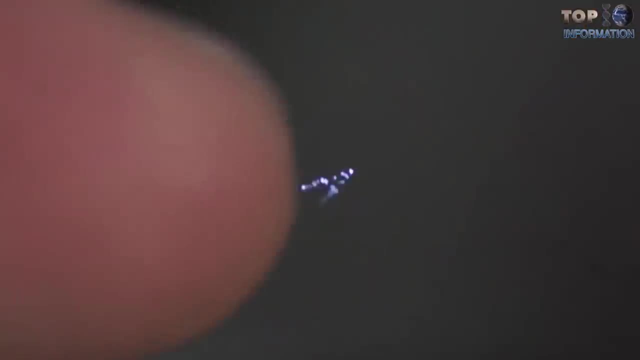 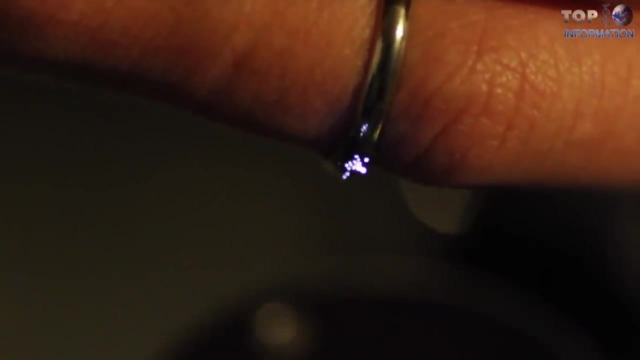 of ionizing air molecules and thus create crackling photon-emitting pockets of plasma. These lights, or voxels, can be arranged in mid-air to create moving floating interactive images. Another portable holographic device is Digital Holographic Table. This is the most complex holographic 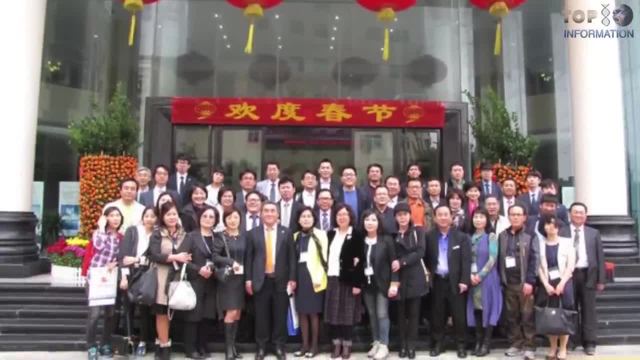 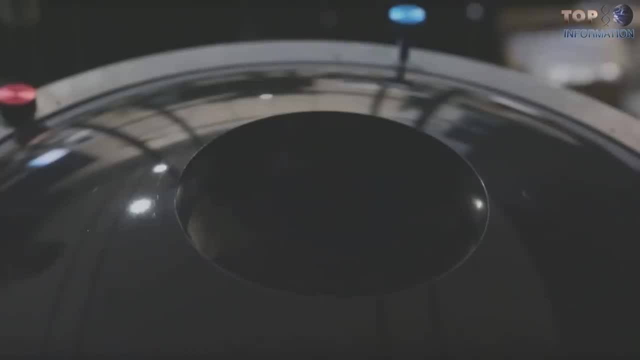 tabletop that is developed by a company, Giga Korea, in collaboration with other businesses and investors. Fortunately, it can produce the world's first 360-degree hologram, and it can be viewed from any angle Thanks to a series of high-powered multi-color lasers. 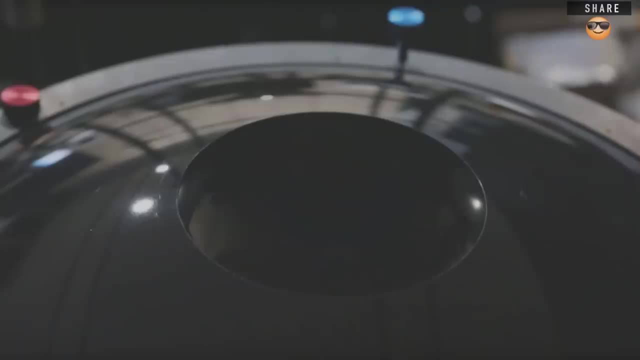 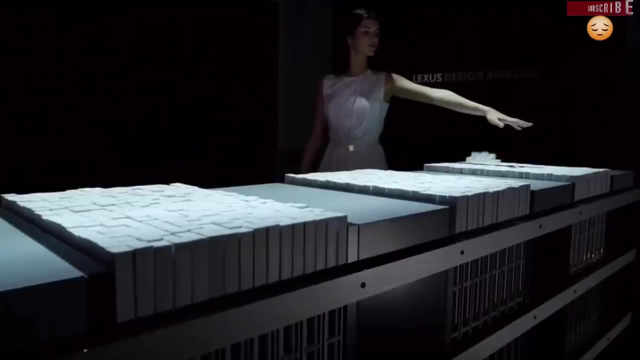 this complex Rubik's Cube projection in mid-air is possible. Number 7: Physical Hologram. Physical holograms are more sophisticated than physical holograms. They can be used to make a real-world object and they are integrated in a way more interactive. Two MIT students. 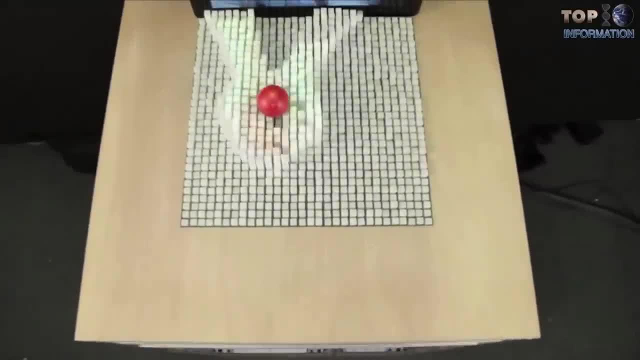 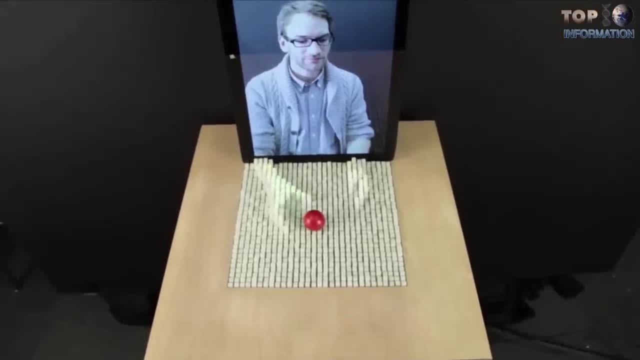 Daniel Leithinger and Sean Falmer invented this complicated and tangible in-form dynamic shape display. It is more advanced than a hologram because it expresses 3D physical telepresence due to the ability to render the shapes of people and objects. So you? 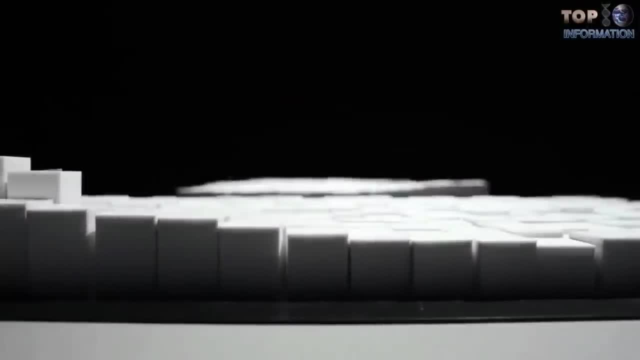 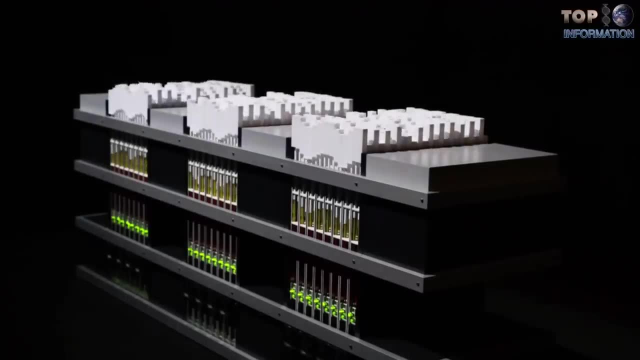 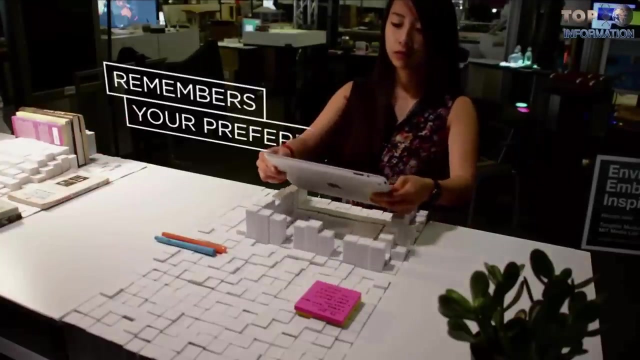 are wondering how it works. In simple words, this table was built with motors, linkages and pins that can render a person physically in real time via a digital source. It is almost science fiction type quality. That's 900 pins each a half inch wide, with 900 separate motors. 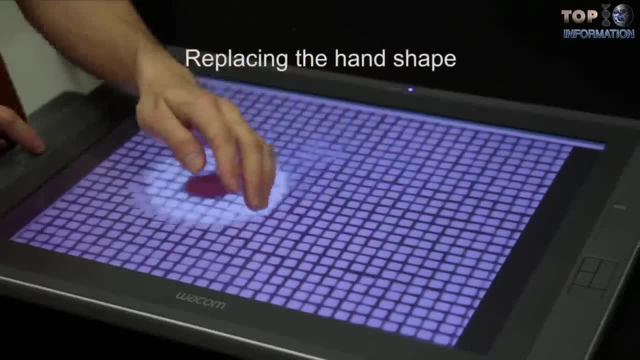 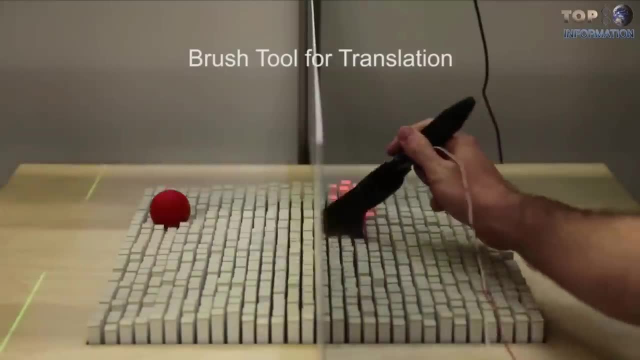 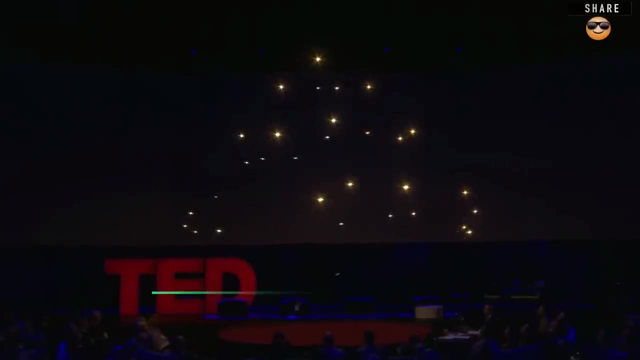 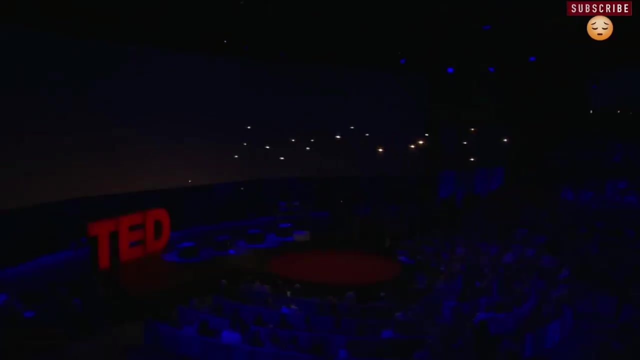 Getting 900 motors in such a dense area was a real challenge. CrazyFly's 2.0 is another physical hologram which uses hundreds of autonomous drones with LED lights. These drones fly in a coordinated manner and are able to express 3D glowing holographic structures. 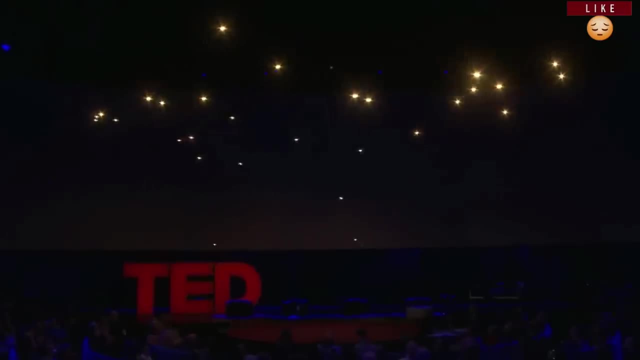 in the air. These are alternatives to the fireworks and the best way to combat air pollution, Designed by Rossi. CrazyFly's 2.0 is another physical hologram which uses hundreds of autonomous drones with LED lights. These are alternatives to the fireworks and the best way to combat air pollution. Designed by Rossi. CrazyFly's 2.0 is another physical hologram which uses hundreds of autonomous drones with LED lights. These are alternatives to the fireworks and the best way to combat air pollution. Designed by Rossi, CrazyFly's 2.0 is another physical hologram which uses hundreds of autonomous drones with LED lights. 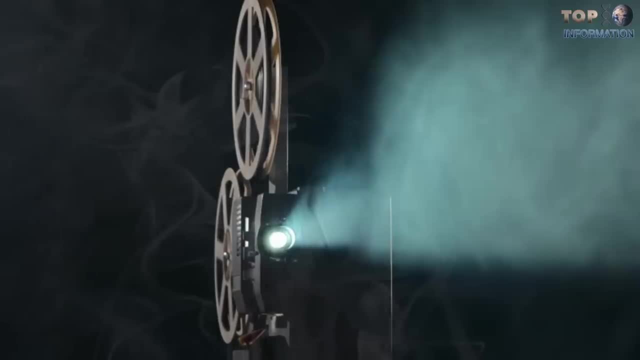 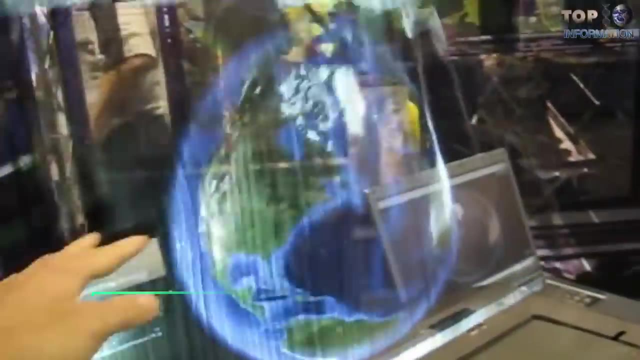 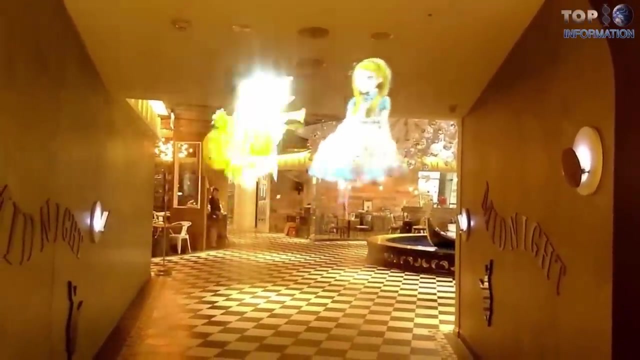 Material Fused Holograms. Material Fused Holograms are those holograms that require a media for its projections. The first example of a material fused holograms is the smoke projector. Smoke projection is an excellent projector technique for holographic effects and low budgets. 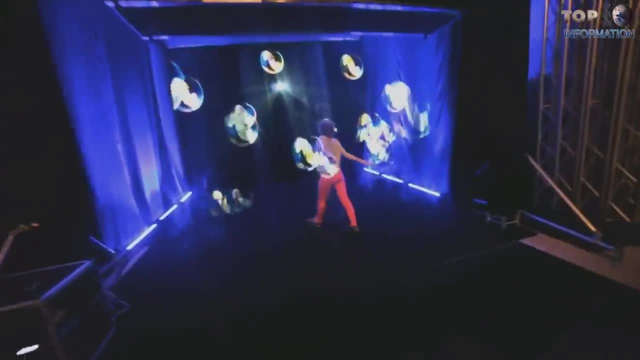 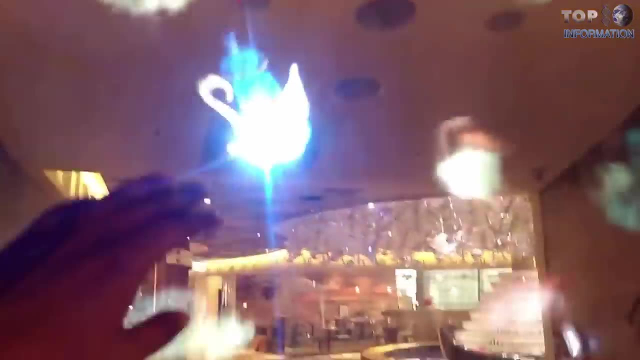 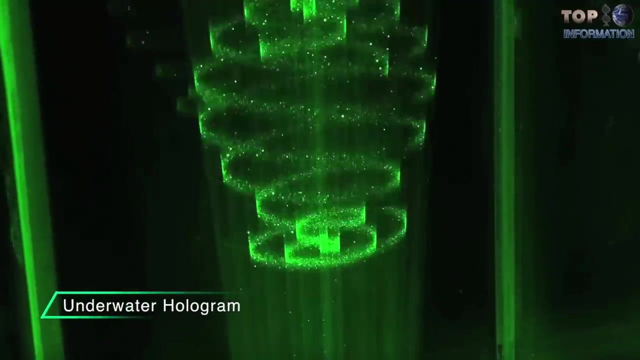 You just need a cool projector and a smoke tube that exhales a continuous, continuous vertical smoke film. It is a really cool and affordable idea to attract customers with this high-tech advertisement. Another example of material fused hologram is Underwater Hologram developed by company. 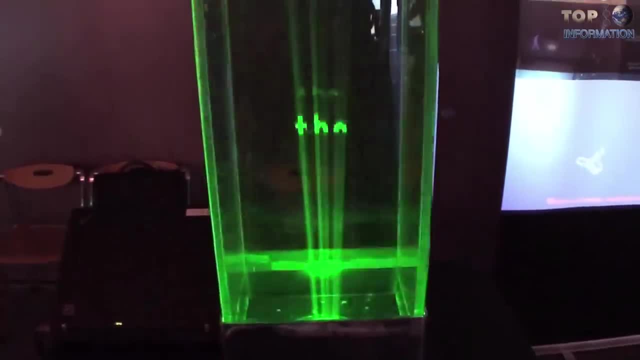 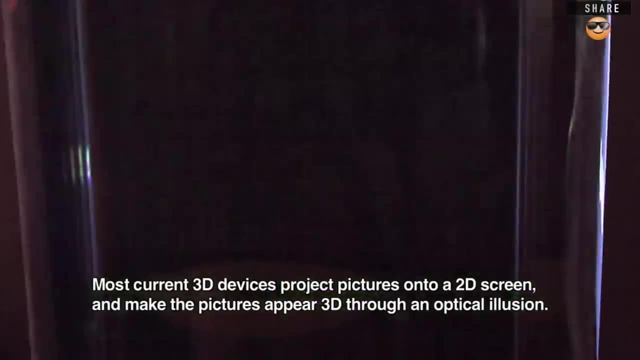 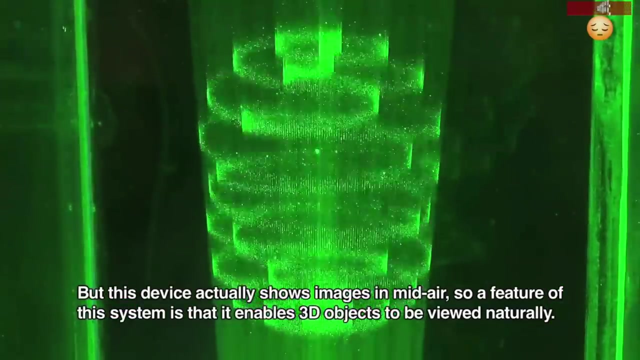 Burton Inc. But you are wondering how it works. These laser lights produce molecular excitation in water to show green holographic patterns. Surprisingly, this system produces 50,000 dots per second at 30 frames per second, which is incredible. 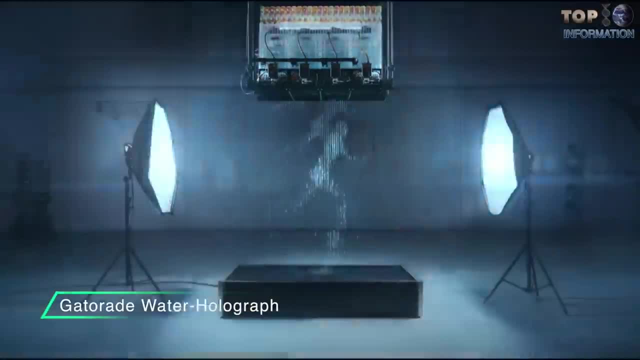 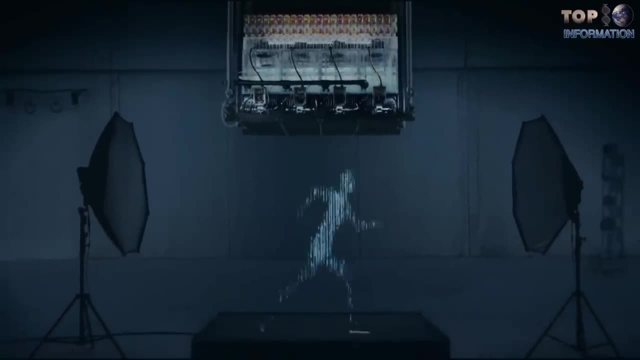 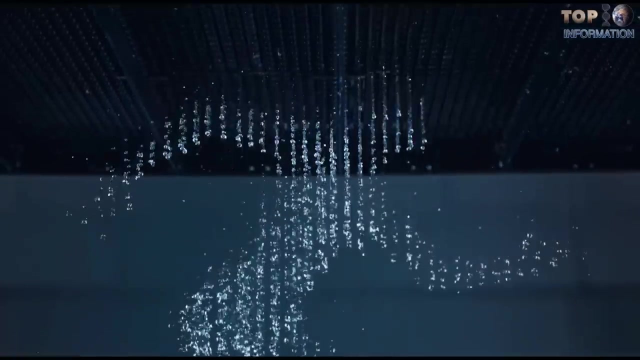 Gatorade Water Holograph is an incredibly creative technique used by an advertisement company, Gatorade. Interestingly, this holographic technology comprises of over 20,000 parts and took 5,000 hours to construct. There are 208 individual nozzles which turned on and off within 2 milliseconds. 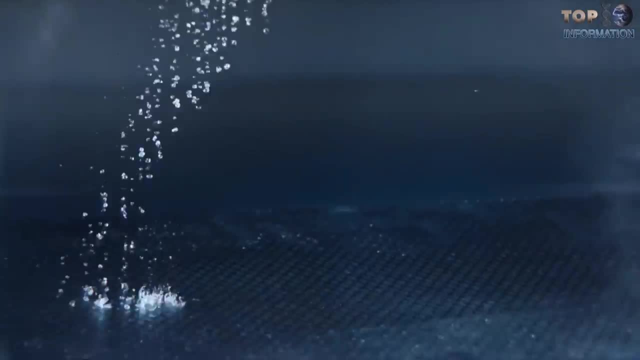 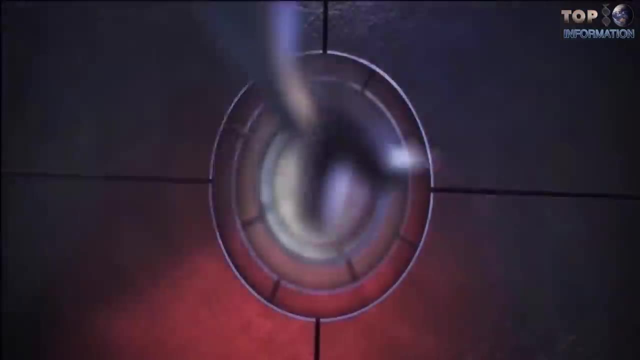 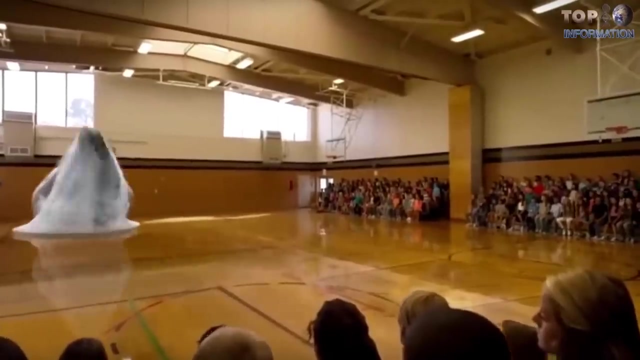 The figure jogs over to a box and starts doing box jumps, with water splashing as its feet hit the box, which is a challenging job to accomplish. Number 5: Holograms for Shopping Malls. It is a 7D holographic technology. 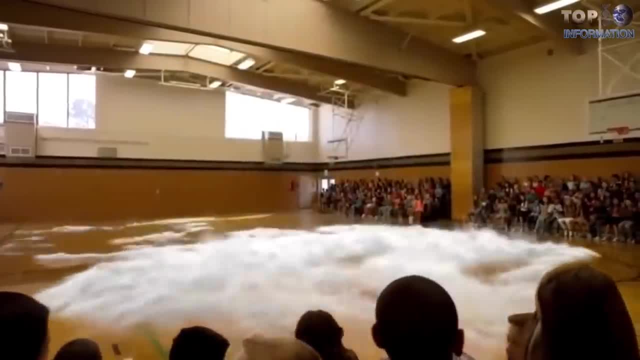 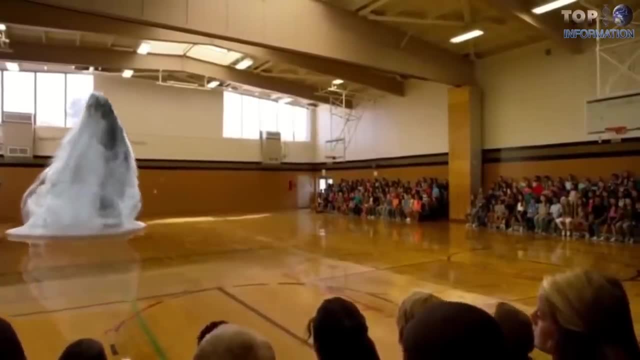 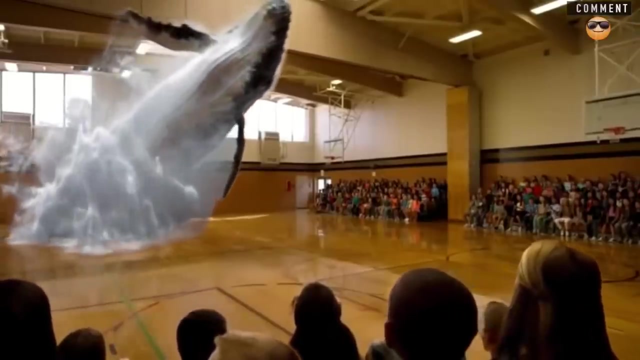 That means it is high-quality holographic captured from seven dimensions with extremely visual effects, As you can see a virtual whale splashing through a school gym floor. That seems to be real, But this technology is still under development. In this concept video released by Magic Leap to show capabilities of 7D technology, 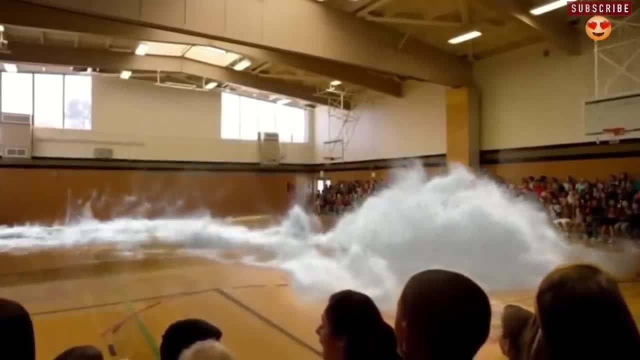 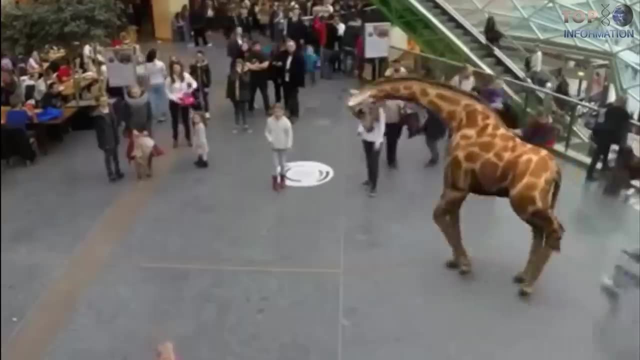 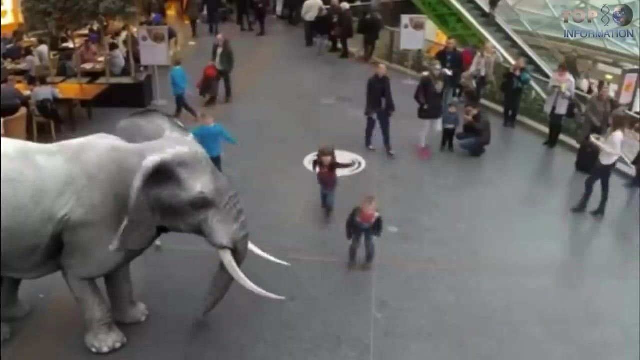 Some videos about 7D technology on YouTube became very viral, like 7D Holographic Show at Dubai and 7D Holographic Zoo at Japanese Mall, where holographic animals like giraffes, monkeys and pandas seem to interact with visitors at Japanese malls. 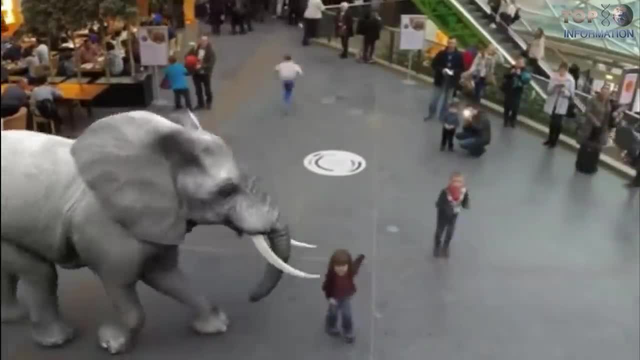 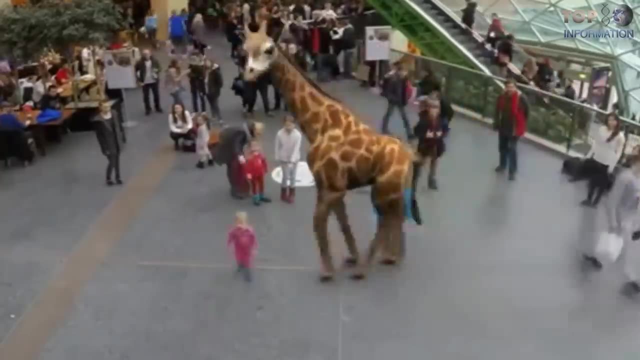 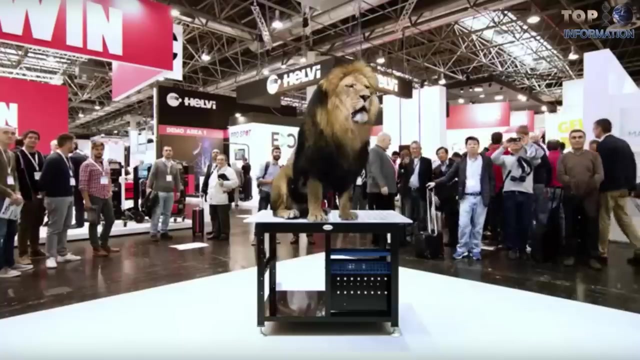 But unfortunately, these videos are apparently a hoax. This video was part of an advertising campaign for National Geographic that became freaking viral, And it was created by using Maya, an animation software. By the way, it is clear that the internet is full of hoax videos, but we can't deny. 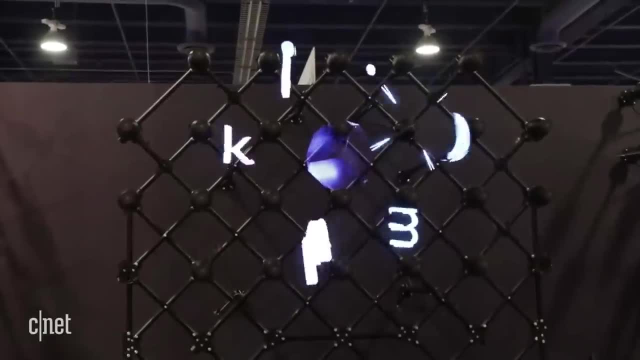 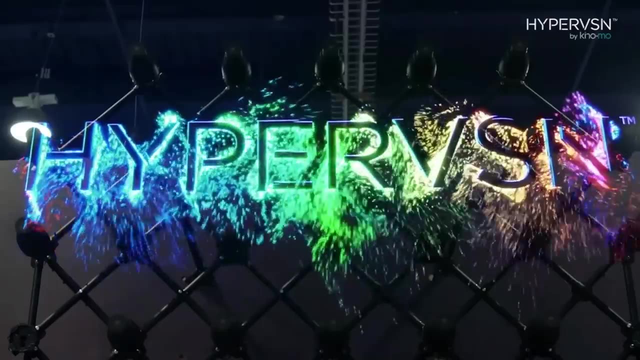 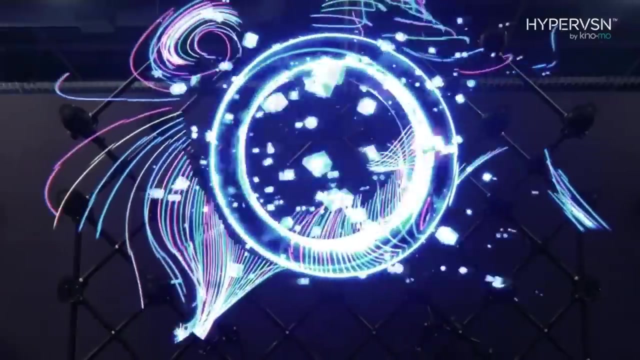 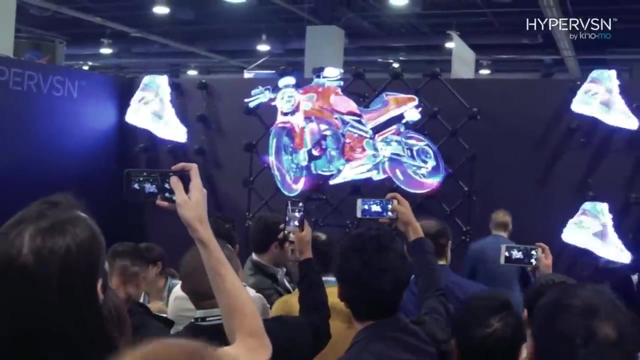 the existence of holographic technology. Another holographic technology is a form of Chinese company, Kinomo. They introduced HyperVisionWall That is capable of producing holographic illusions near to HD resolution. This unique wall consists of so many spinning fans. The sophisticated LED propeller produces holograms based on advanced software algorithms. 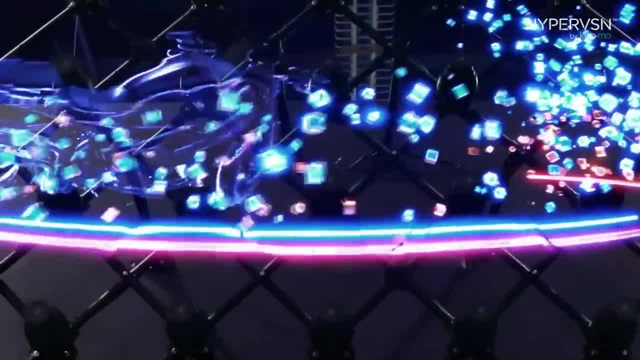 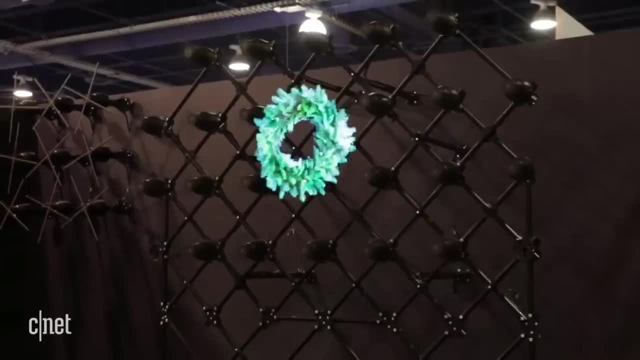 This wall is 3 meters in size and power efficient because it consumes just 65 watts of energy. It costs $3,200. So it's definitely designed for retail, sports venues and commercial displays. Thanks for watching. If you enjoyed this video, make sure to hit the like button and share it with your friends. 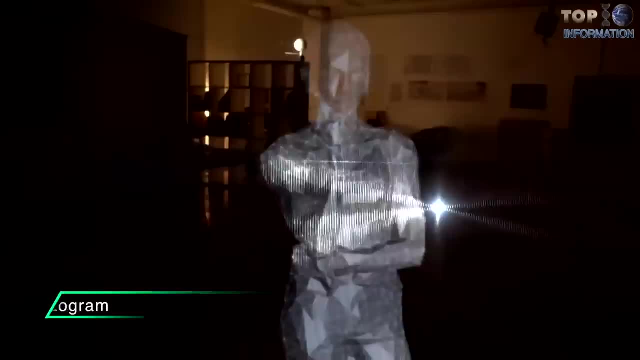 Don't forget to subscribe to our channel for more videos like this, And don't forget to turn on your notifications so you don't miss out on any of our latest videos. We'll see you in the next video. Bye for now. Nologram is a glasses-free and most realistic holograph. 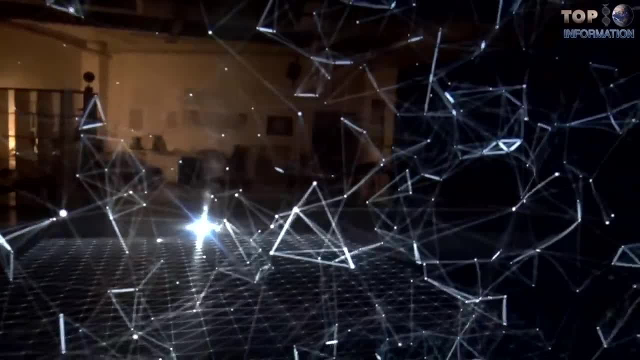 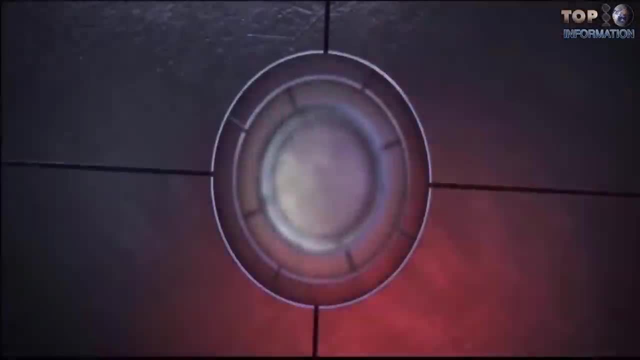 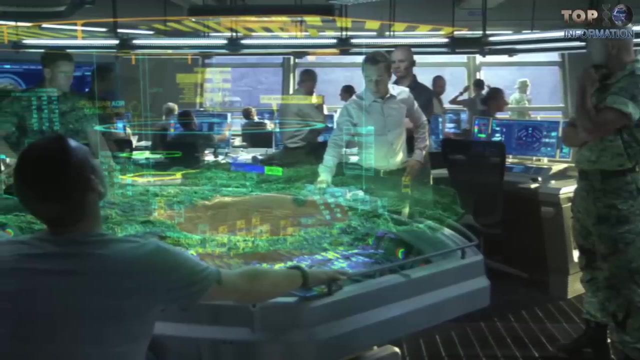 And this new technique, developed by a French artist named Joanie Lemesire, uses two-dimensional projections paired with a motion sensor to make the image appear to be fully 3D. Table Holograms. Table holograms are those holograms that require a table. 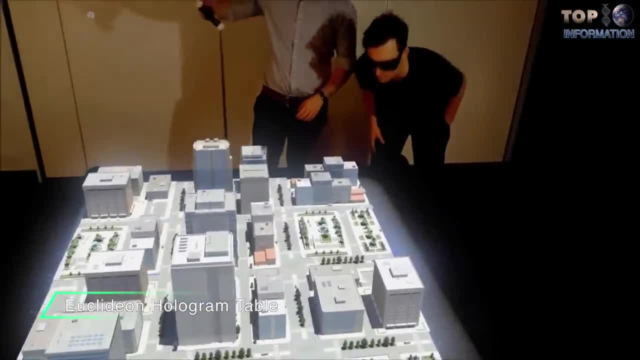 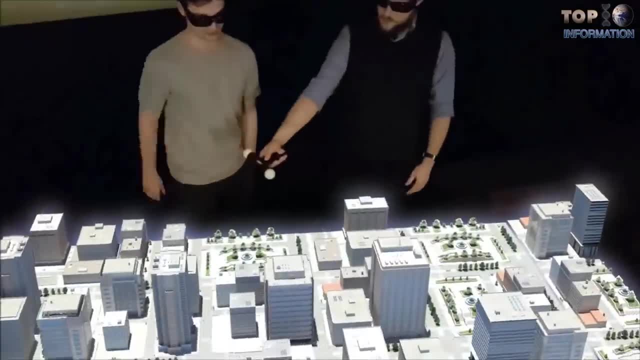 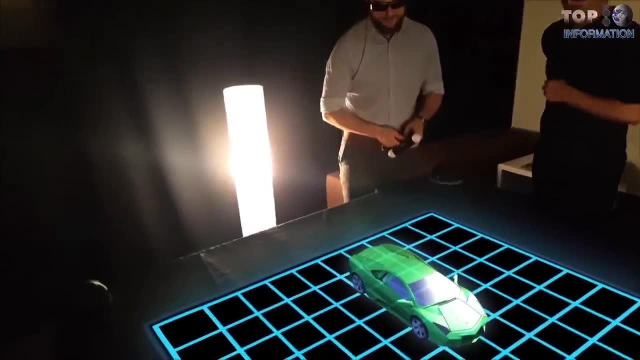 The world's first multi-user hologram table. Up to four people can walk around a holographic image and interact with it. Euclidean Hologram has the great processor and powerful GPU that makes the 3D objects out of light and it can artistically project them. 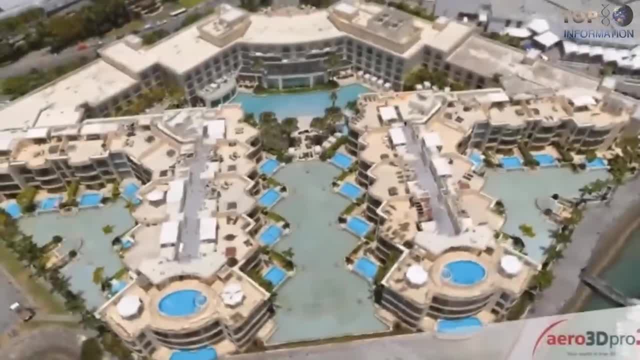 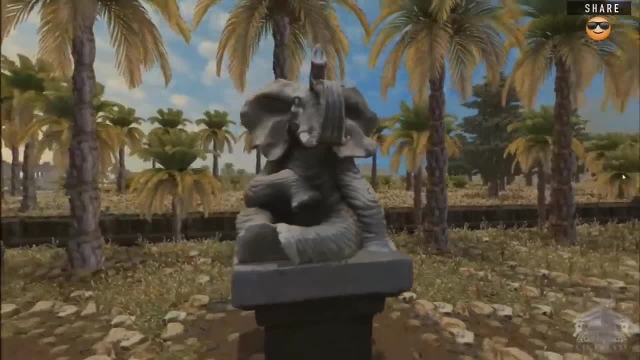 The computer makes these by coordinating little theoretical atoms of light. It can be used to sell real estate off the plan, like used to be done with the world's smallest building models, Or it can be used to view the entire city Or even the whole country. 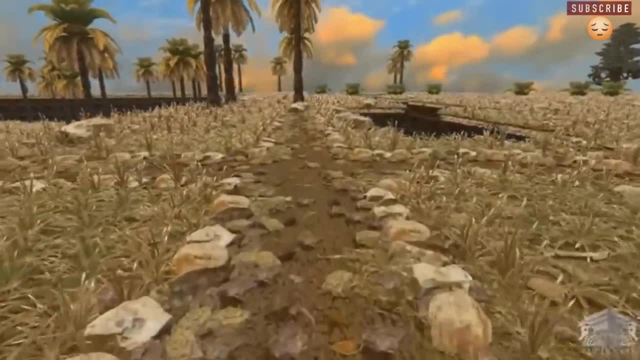 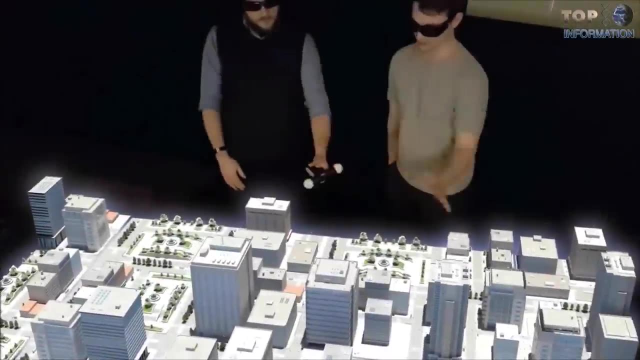 It has the world's most powerful 3D graphics and the most powerful algorithm. This incredible combination helps the table to process 64 atoms per cubic millimeter of data. That is equal to 1 million atoms per cubic inch, to put it simply. 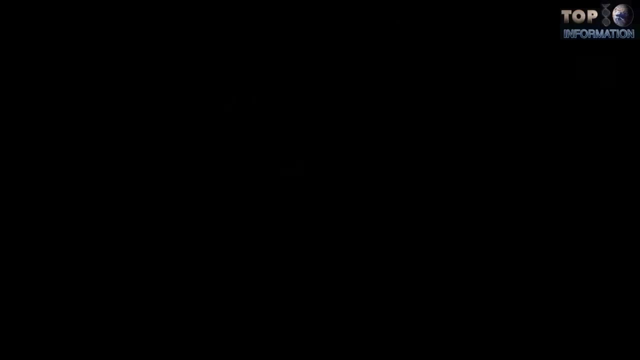 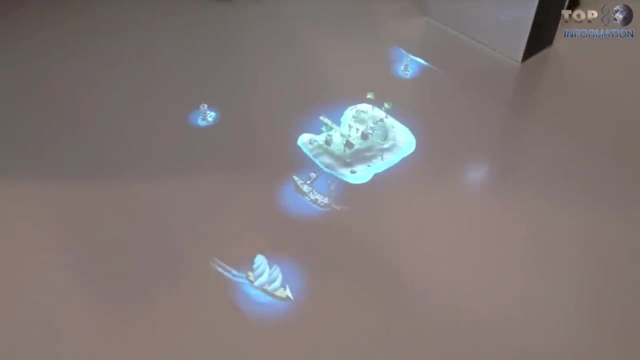 It means that it can handle 1,000 gigabytes of graphical data. Another example of table hologram is Hololamp, the world's first glasses-free portable holographic device. It can also control 3D illusions directly on your table. 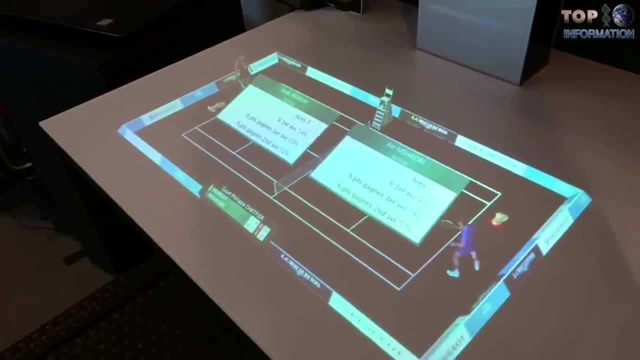 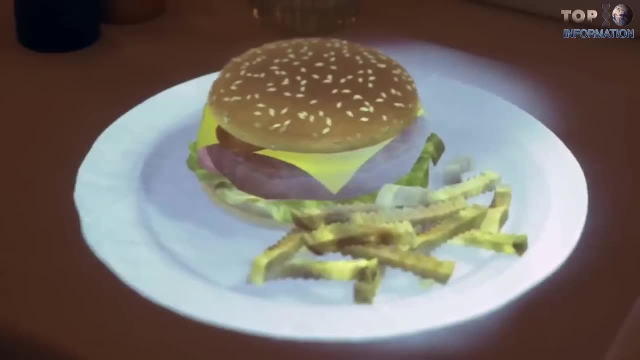 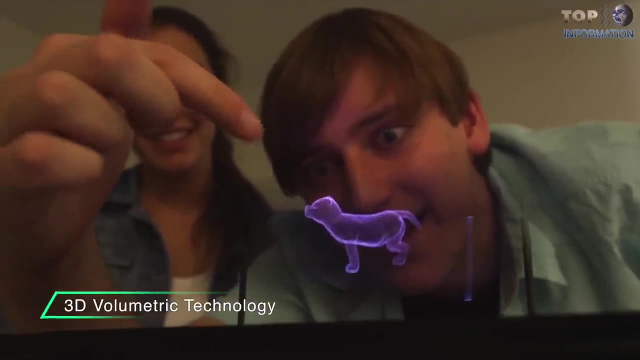 Hololamp applications are made with Unity, which is a leading global game industry software Based on a touch detection technology. Hololamp allows you to control the virtual 3D objects using your hands. Another table holographic device is 3D volumetric technology, which brings digital content to. 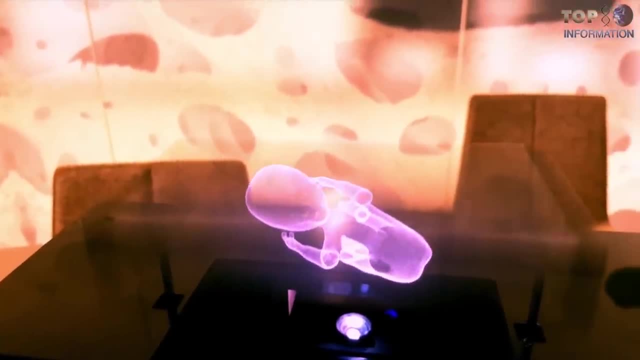 life and helps to empower people to visualize, communicate, learn and experience the world. Hololamp is a powerful device that allows you to control three-dimensional objects by using your hands. The Hololamp application can be used by computers, computers, computers or computers. 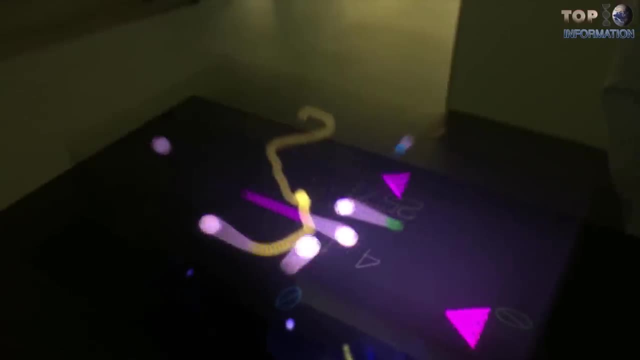 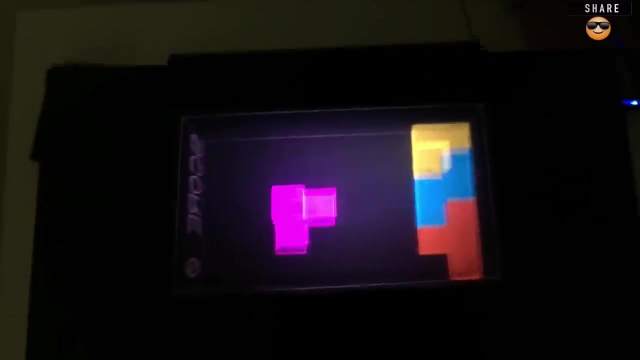 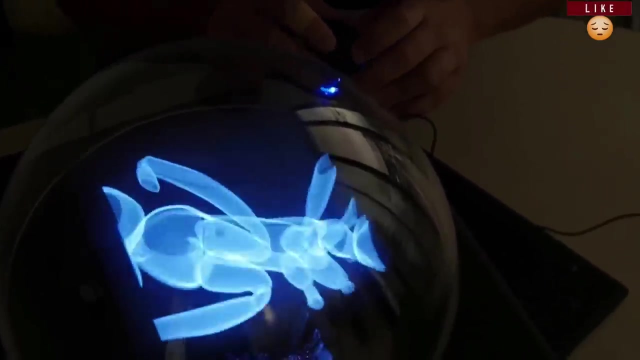 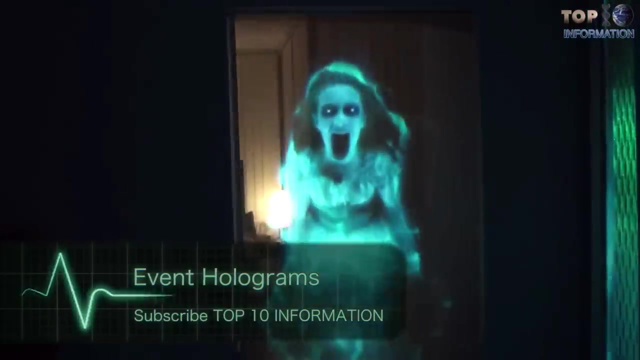 collaboratively, have fun with no barrier to the 3d experience. no special glasses are required. it is a way more interactive with 3d awesomeness, allowing for multi-user and real-time interactivity- a socially engaging way to use technology for entertainment. number three: event holograms. event holograms. 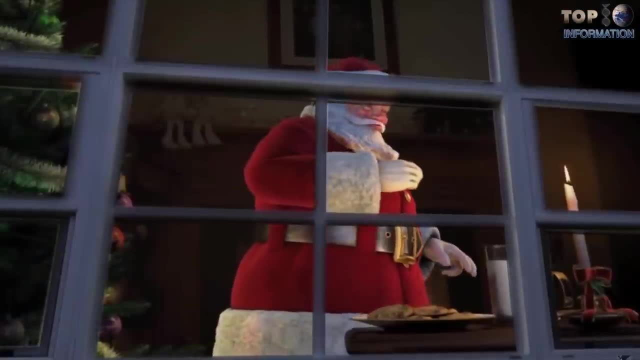 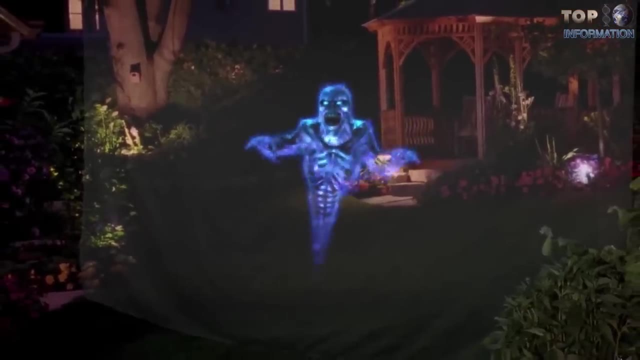 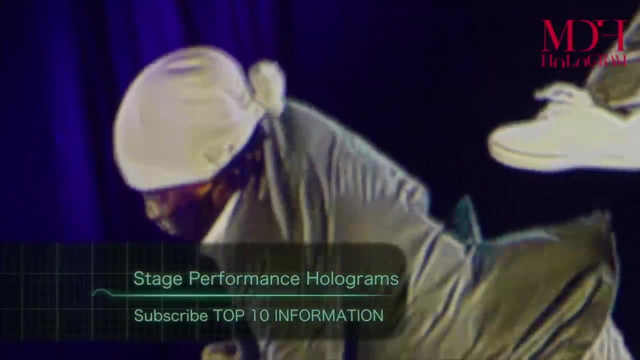 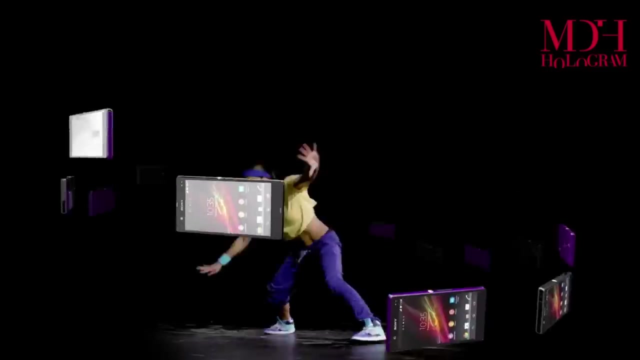 are holographic projection technologies that is best used for Christmas celebrations or it may be used in Halloween to have some fun developed by company at most effects. number two: stage performance holograms. MDH hologram is pioneering in the holographic technology industry and is the world's leader in. 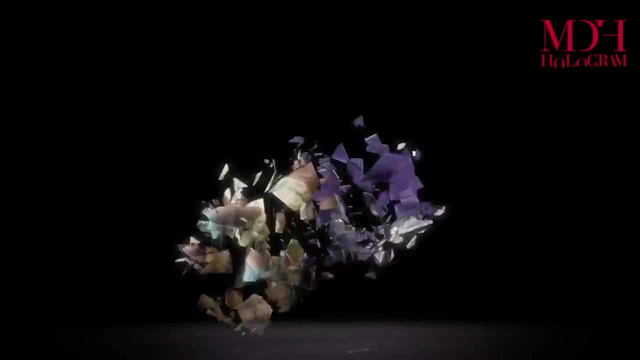 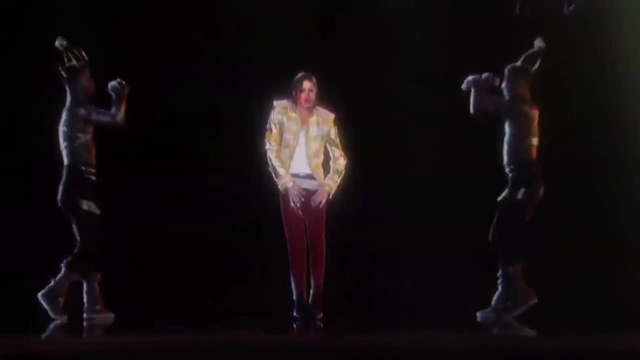 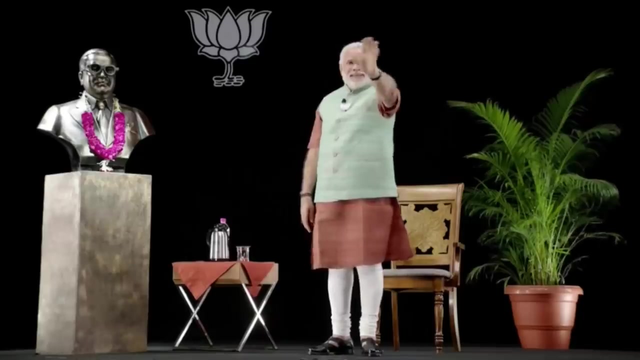 holographic technology. MDH hologram is the most advanced holographic technology in the world technology that are mostly used for stage performances and best preferred by singers, actors, magicians, politicians and corporations. the best example of using this technology is the recent victory of Indian Prime Minister, Narendra Modi. he 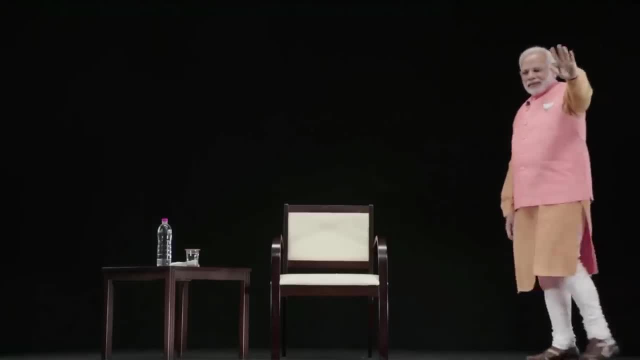 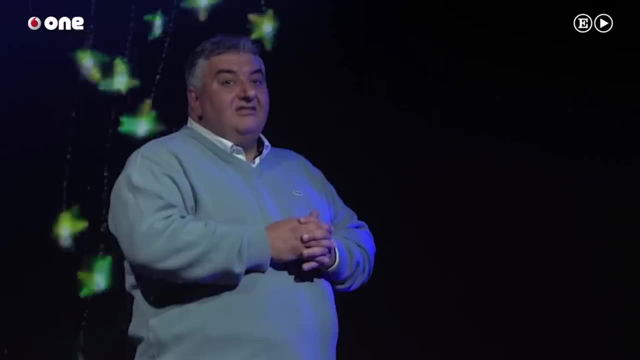 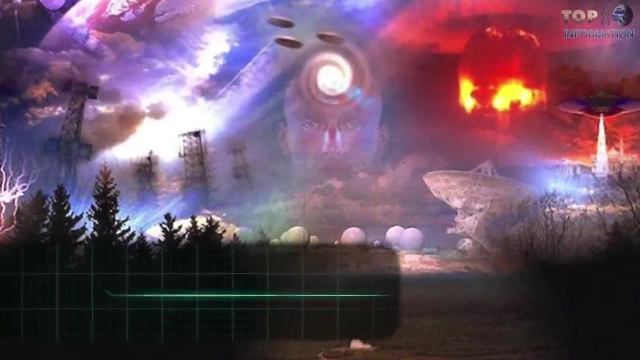 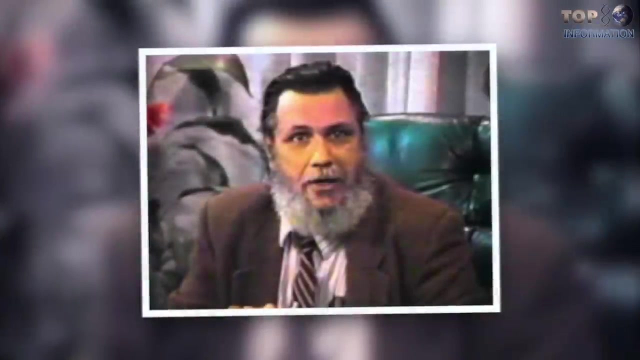 used this MDH holographic technology to simultaneously broadcast himself in various states of India. but this technology is not cheap. it's pretty expensive. number one conspiracy hologram. the best example of conspiracy hologram is the project blue beam. this conspiracy theory was first proposed by two Canadian journalists. 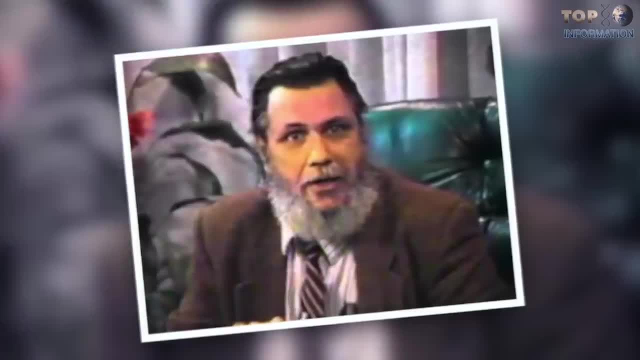 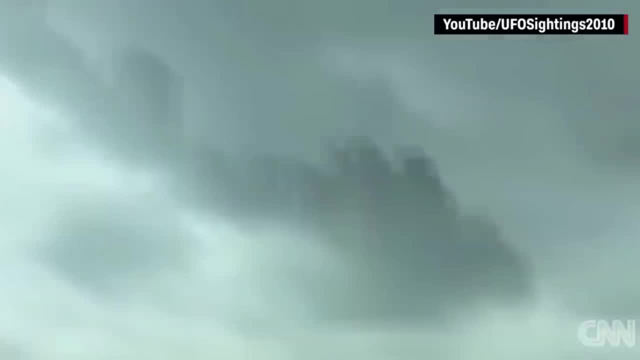 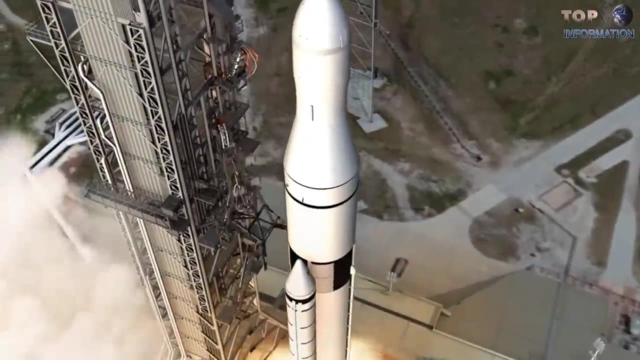 Cuba soy and Serge Monast in 1994, after two years, mysteriously both died due to heart attack. if you remember the event where the dark floating skyscrapers appeared within clouds above China, then you are all well aware of this conspiracy theory. NASA launched four holographic satellites that were used to 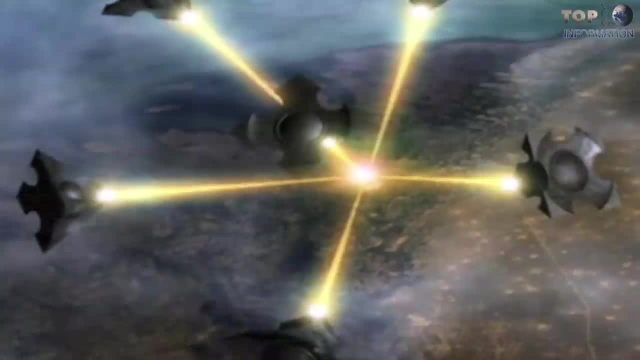 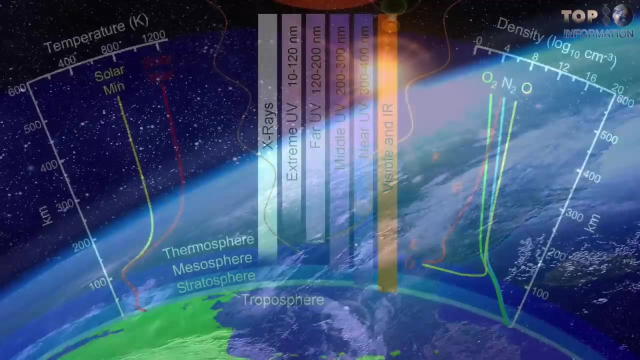 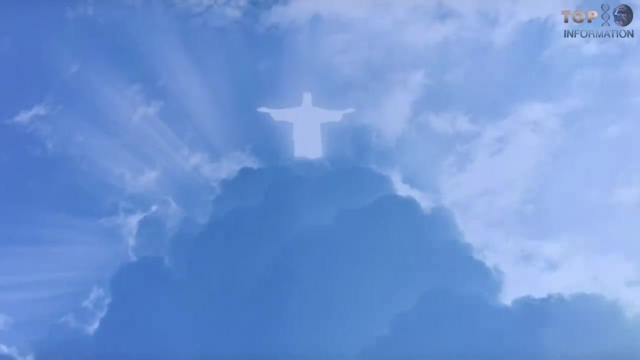 produce holographic images by simultaneously focusing on a single region of the earth. how will it work? the answer is that the holographic laser beam can ionize air molecules of a particular region so that local people will be able to see the hologram. this conspiracy claims that NASA is attempting to 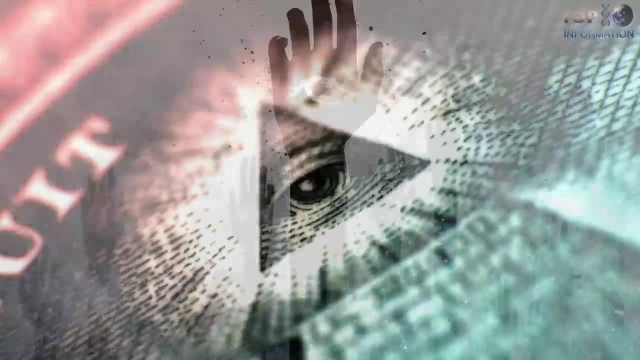 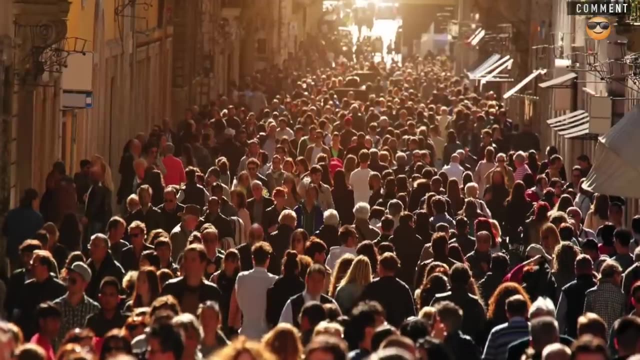 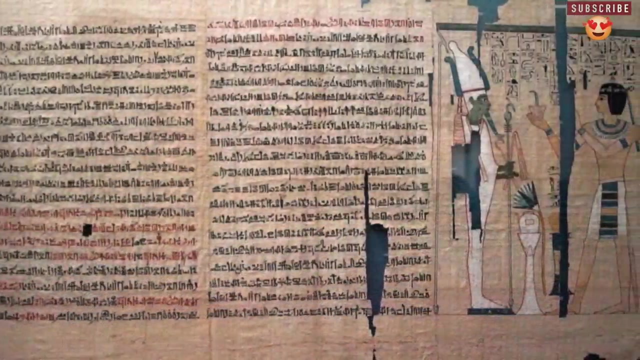 implement a new age religion with the Antichrist as its head and start a new world order via a technologically simulated second coming. this secret mission wants to control the entire population with fears of alien attacks by misusing religious prophetics and archaeological knowledge of all. 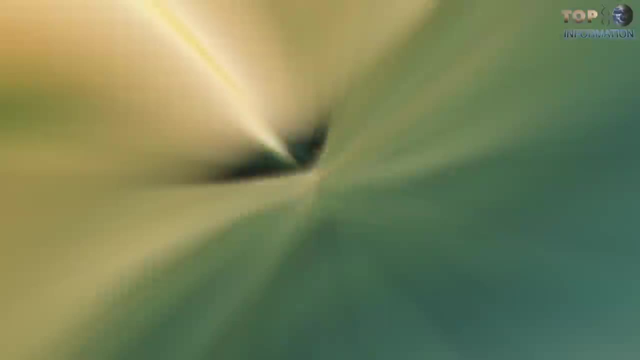 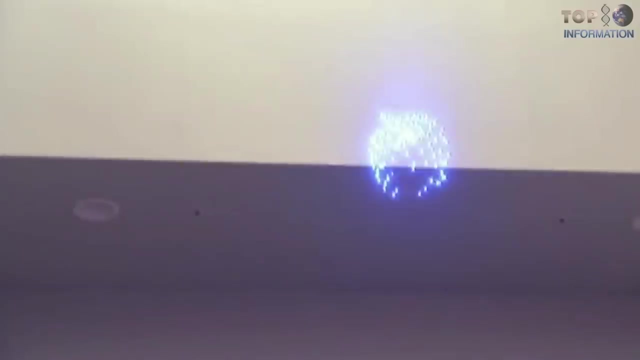 dominant faith. if this technology is real, then it should be number one on our countdown list. thanks for watching. which technology did you find the most interesting? tell me the reason in the comment section. if you are new here, then feel free to subscribe. share this video with your friends and don't miss our